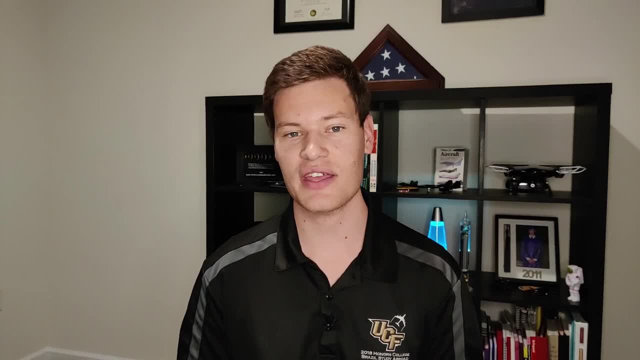 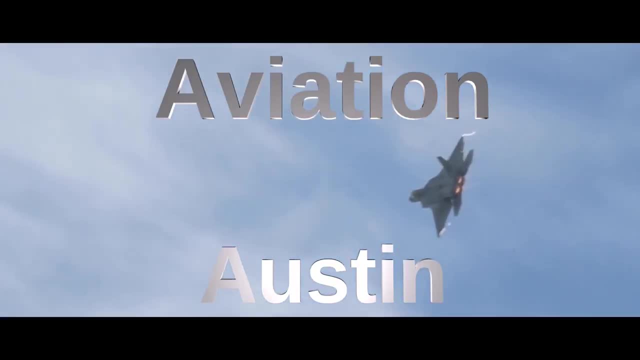 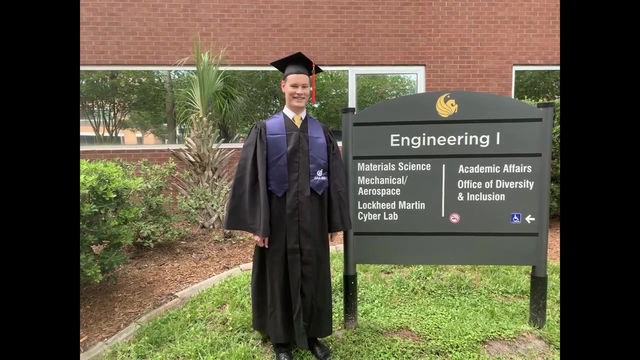 by step, all the way from high school, what the best path is to becoming an aerospace engineer. Intro: While preparing this guide to becoming an aerospace engineer, I drew on my own experiences as an aerospace engineer, as well as the experiences of my colleagues and classmates. So let's go ahead and jump right into the guide. So if you're still in high school, you want to. 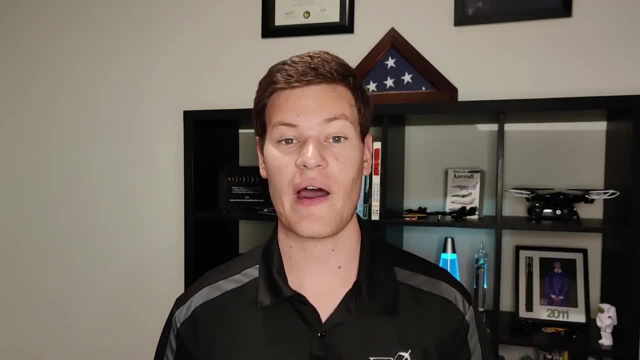 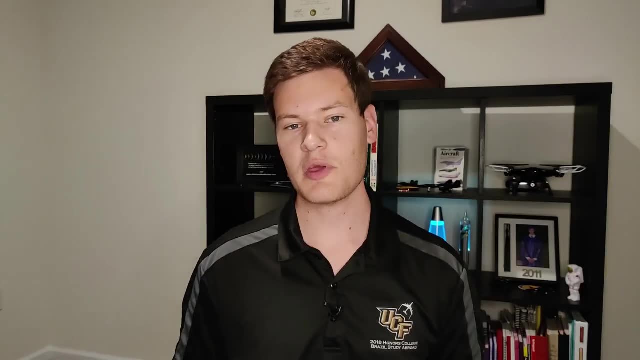 focus on your math and physics courses. This is going to help you feel out whether or not you want to become an aerospace engineer, because becoming an aerospace engineer requires a lot of math and a lot of physics. Now, me personally- actually, I've been doing a lot of math and physics since I was in high school. 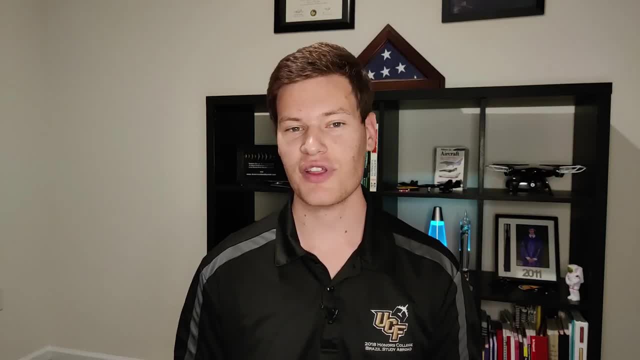 I actually didn't enjoy my math classes in high school that much, but I really loved physics and what I started to realize was physics is really just the application of math in real world scenarios and I really like that and really, in essence, engineering is just applying math. 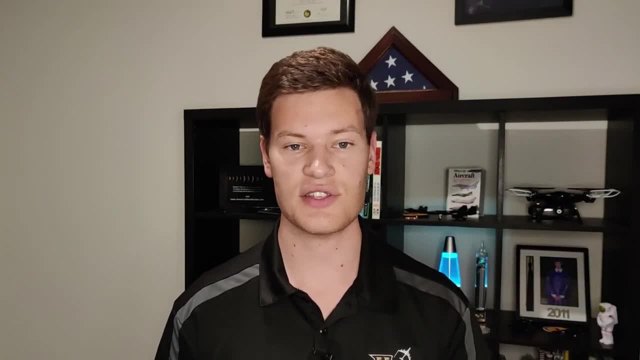 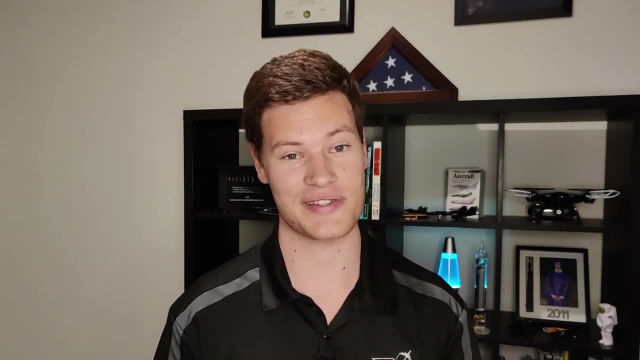 to real world scenarios. So if you've taken and enjoyed these classes and you want to pursue an aerospace engineering degree, the next course of action I would suggest is actually not the conventional wisdom, But I would actually recommend that you don't go to a traditional four-year. 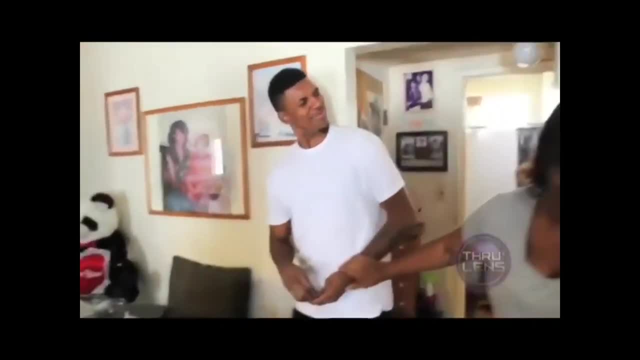 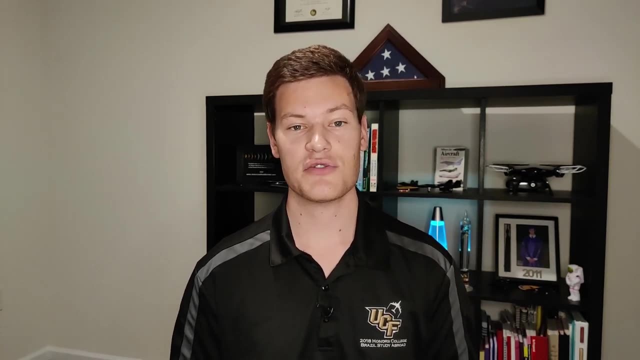 university. You don't go to a university that's a four-year university. You don't go to a university right out of the gate. What I would instead recommend is that you go to a community college or a local state college and pursue an associate's degree, Taking classes at a community. 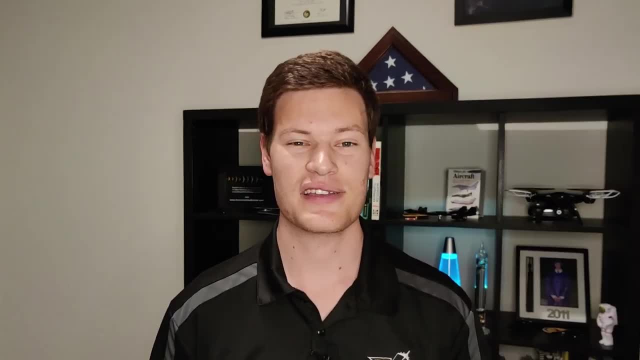 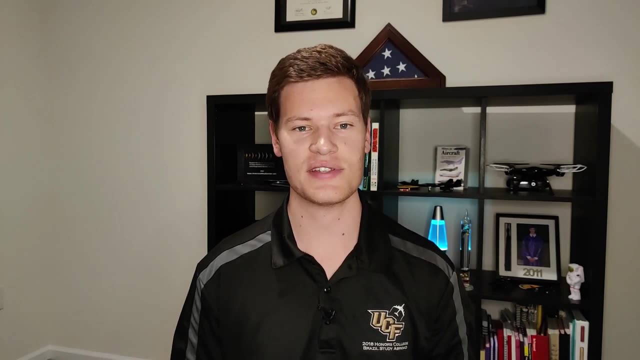 college is a great way to ease yourself into an engineering degree, because an engineering degree is an incredibly rigorous program. So no matter what engineering program you're going to go into, you're almost guaranteed to have to take calc one, two and three differential equations- at least one. 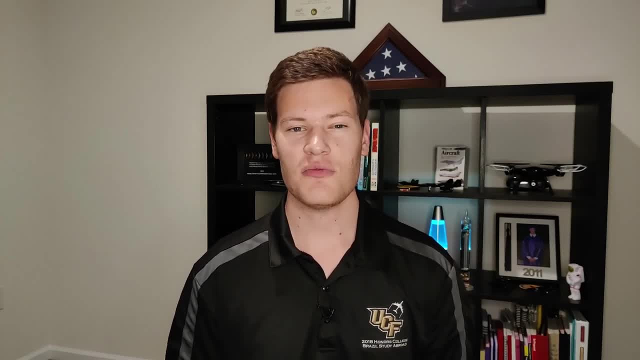 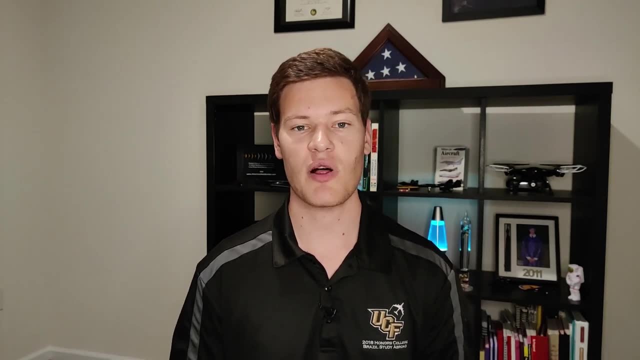 chemistry, physics one and physics two, and you might as well take those at a community college, where you're going to have better individualized help from a professor if you need it, and smaller class sizes so you'll be able to speak up if you ever have a question in class. A lot of those you 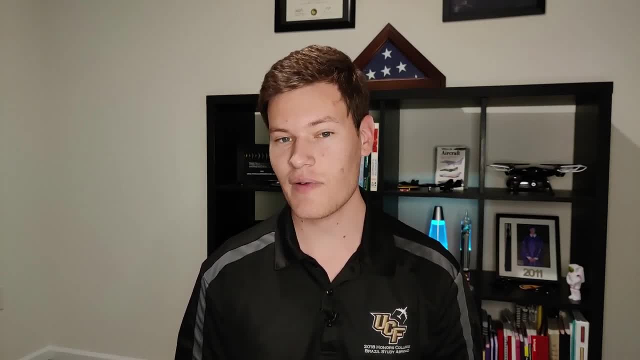 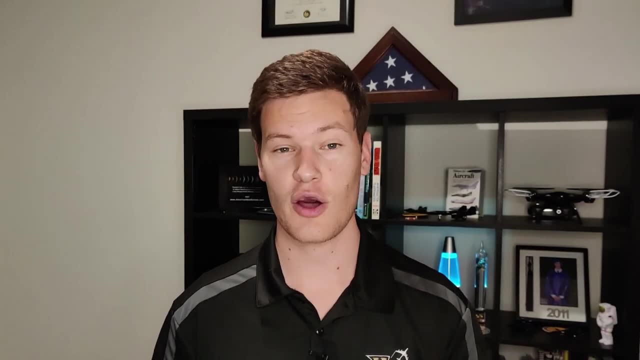 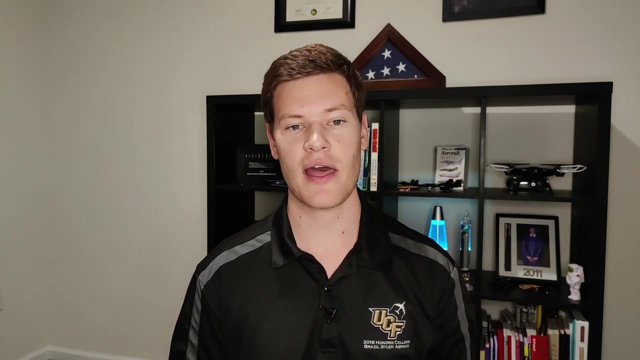 don't get the opportunity at big universities, and I would especially recommend going this route if you're going to be personally paying for your college. Another reason I strongly recommend going to community college before a traditional four-year university is because it's so affordable. So, whether you're paying for your own university or not, going to community college is. 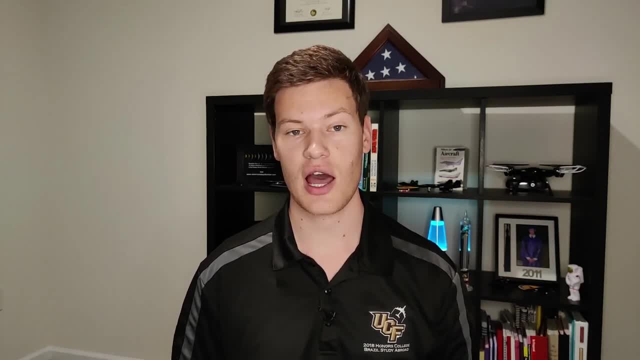 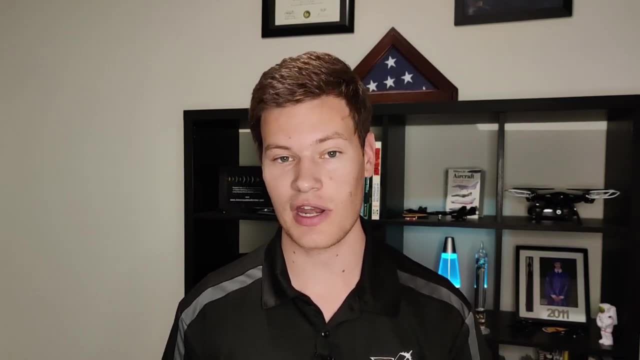 really going to allow you to be able to work on the side, maybe a part-time job, or, if you choose not to work during this time, you're not going to have to take as much loans out or, just frankly, pay as much if you already have the money. In fact, when I attended community college myself, most 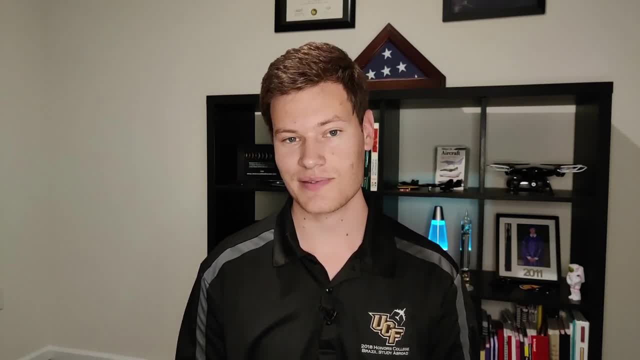 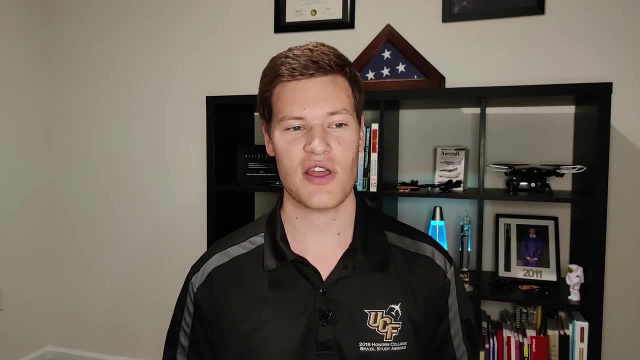 of the tuition was covered by federal income based grants. and my final reason for advocating going to a community college before going to a traditional four-year university is because if you graduate from a four-year university, you're not going to have to pay for your tuition. This is the only way. 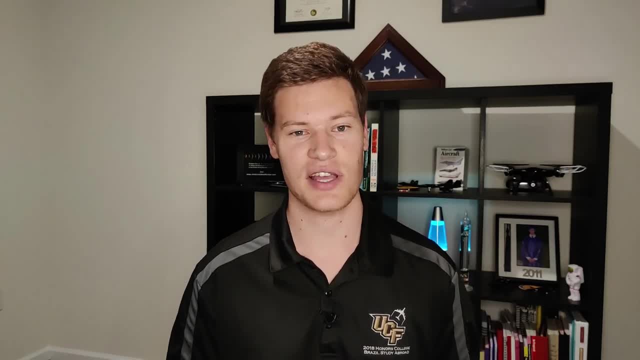 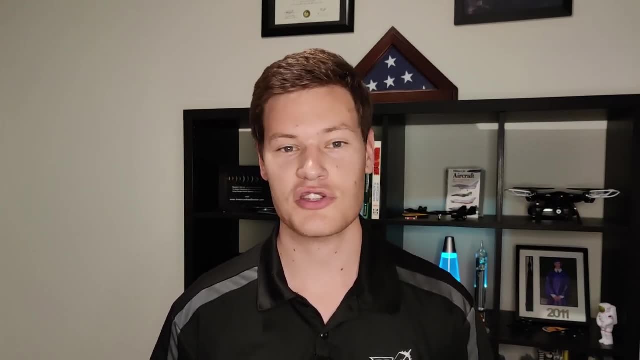 university with a bachelor's degree. it's not going to have an asterisk that says, oh, but he attended a community college. it doesn't matter, it's still going to say the name of the big university that you go to. so there's no shame in going to the community college. so there really. 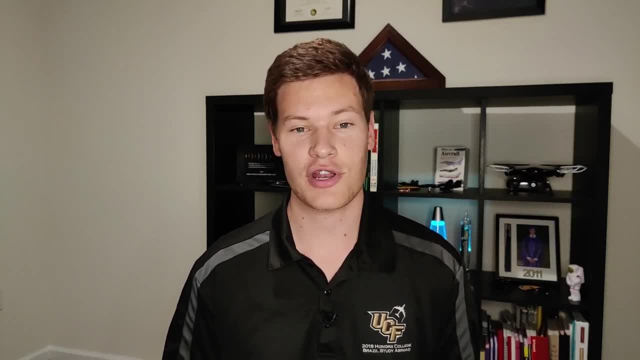 isn't any financial or educational reason why you shouldn't go to a community college before you go to a four-year university. and for some universities it's even easier to transfer than it is to go from high school straight into the university. and this leads us to our next point: selecting an aerospace. 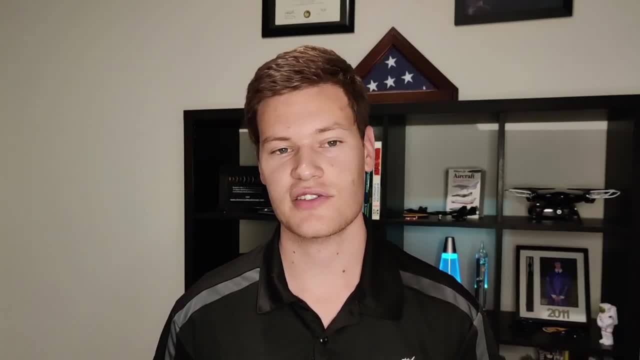 engineering program. now here. of course, there's no shortage of factors, of what you need to look at when you're selecting university. obviously, price is going to be a huge factor if you're paying for college yourself, but there's a few things i need to make sure that you're looking. 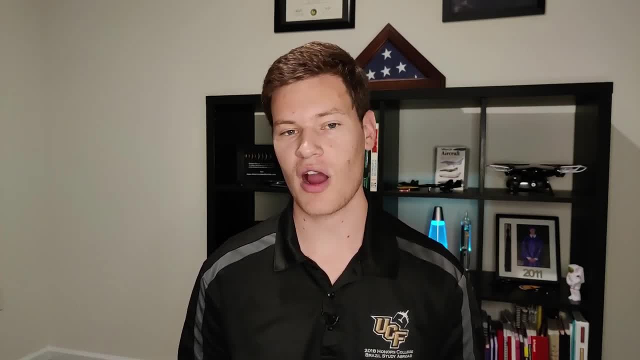 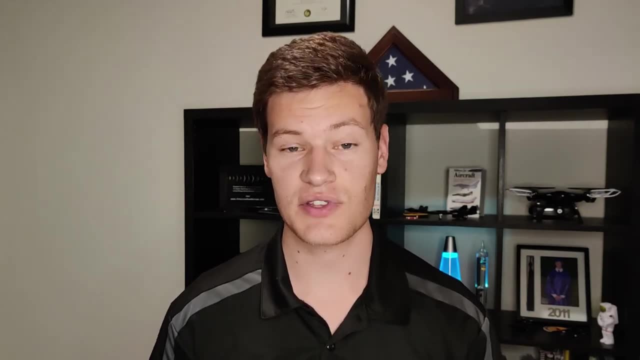 for when you're looking into universities, the first, and probably more obvious, is you need to make sure that it actually has an aerospace engineering program, and one thing you need to make absolutely certain that you check on is to make sure that your program is abet accredited. 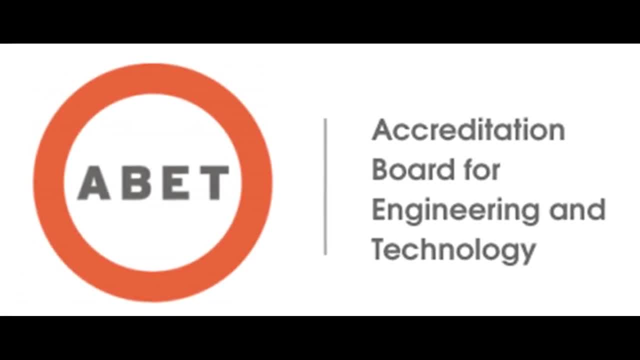 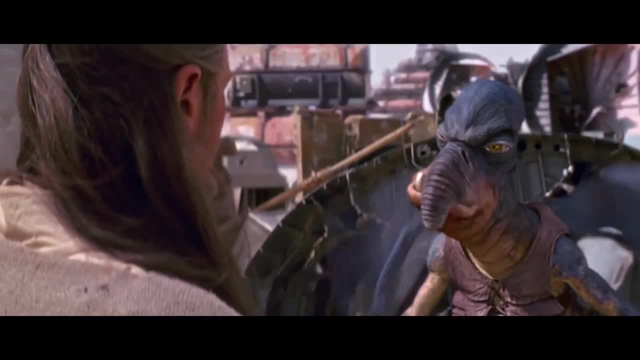 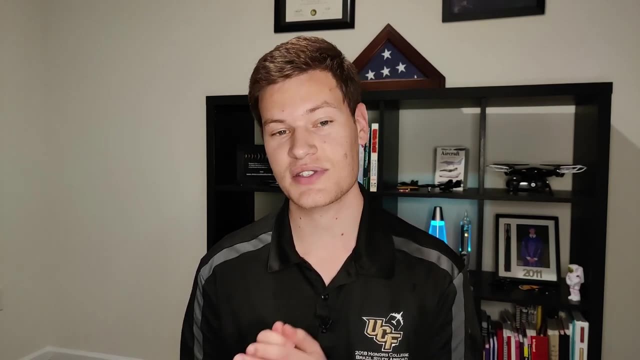 if you don't graduate from a program that is abet accredited, your degree means nothing. your credits will not transfer to another university credits will do fine. no, they won't. you won't get hired for a job because you didn't go to an abet accredited school, so you need to make absolutely certain that you go. 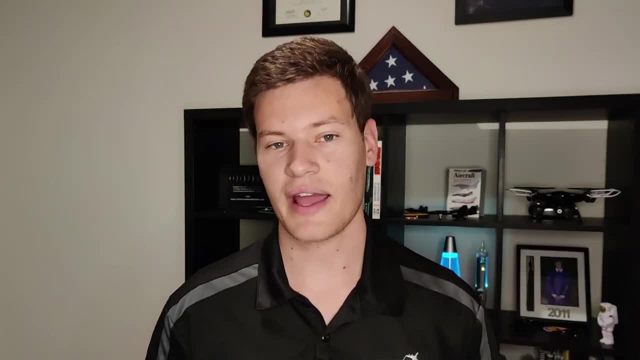 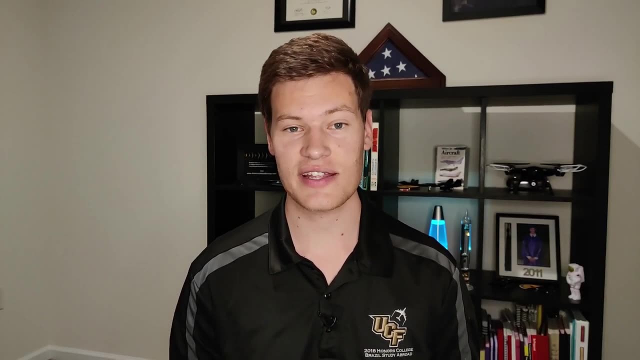 to an abet accredited aerospace engineering program. now, like i said, not all universities offer aerospace engineering, so if the school that you're looking at does not have aerospace engineering and you're dead set on being an aerospace engineer, what you can do instead is mechanical engineering, mechanical engineers and aerospace. engineers take almost the exact same classes for at least the first three years of their program. the only real difference between a mechanical engineer and aerospace engineer is that aerospace engineers take more aerodynamics focused classes, for example fundamentals of aerodynamics, high speed aerodynamics and propulsion systems, but essentially mechanical engineers just. 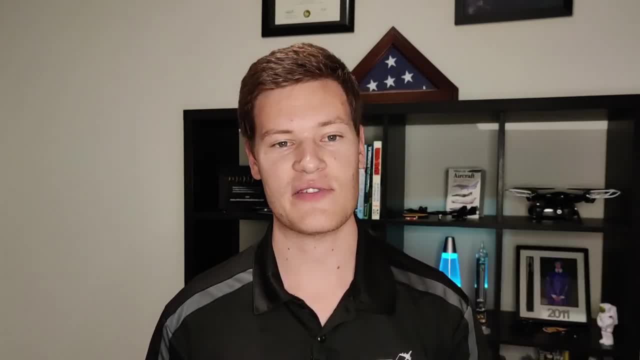 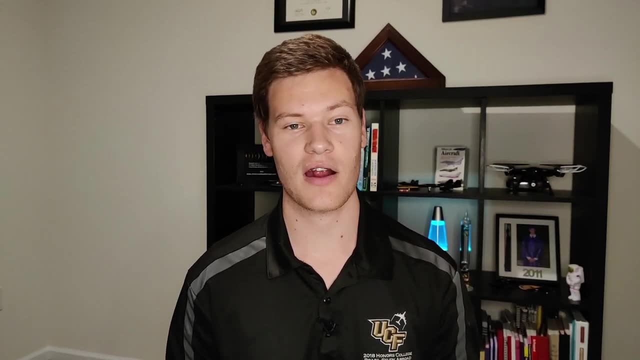 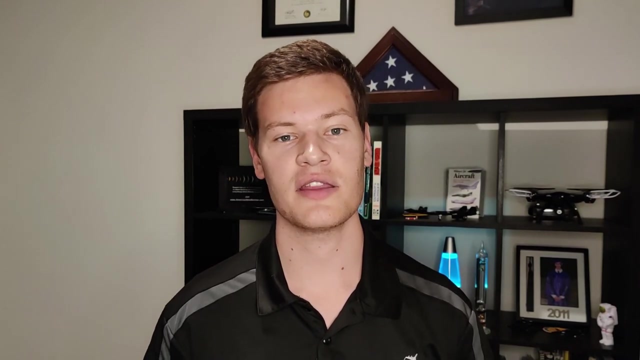 have more opportunities to take more electives and don't have as many required aero classes. in fact, they're so similar that almost all hiring engineers, when they're looking for aerospace engineers, will hire aerospace engineers or mechanical engineers almost interchangeably. so don't stress too much of the university that you're dead set on doesn't have aerospace. 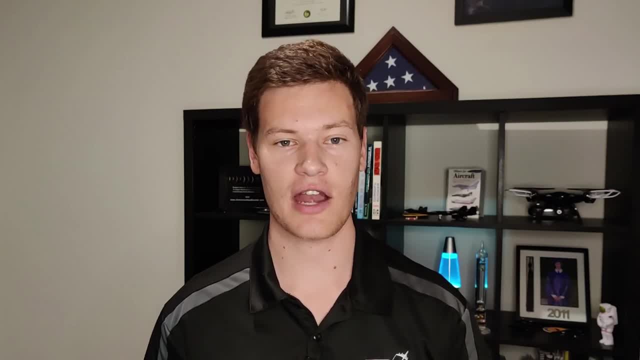 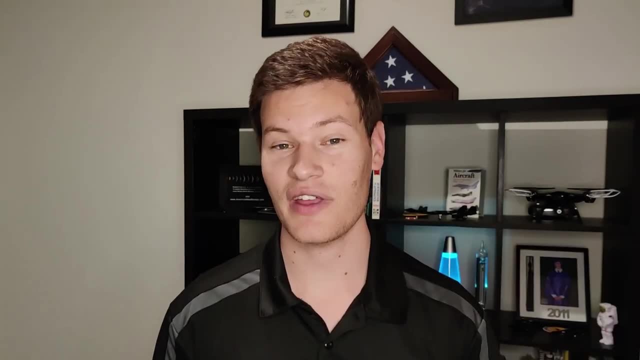 engineering as long as they have an abet accredited mechanical engineering program. so you finally made it to your four-year university and you're in your aerospace engineering program. what's next i really have to warn you about engineering is incredibly difficult. if you're, aerospace engineering program is anything like mine was. you're going to be pushed to your limits- a typical 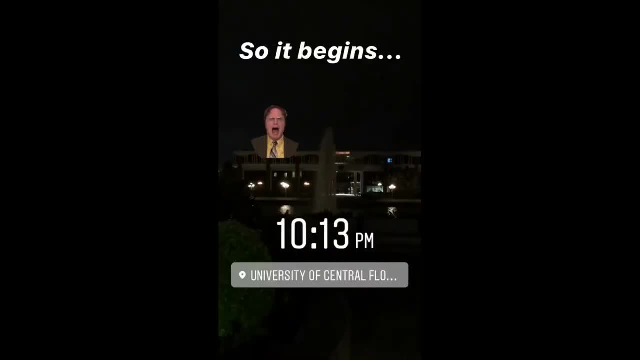 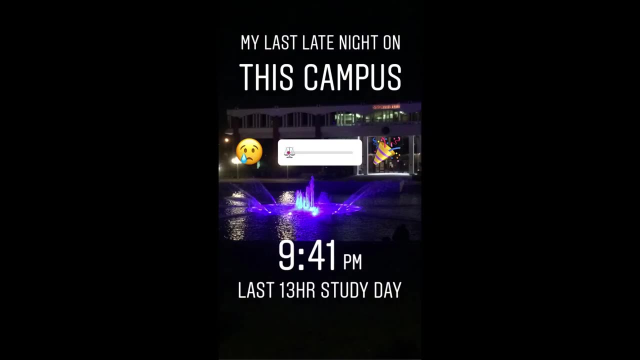 day. as an engineering student, you're going to be studying at least eight to ten hours a day, and that does not include finals, midterm season. so i have a couple tips that were essential to my survival in an engineering program. my first and foremost step that i would tell any: aerospace. 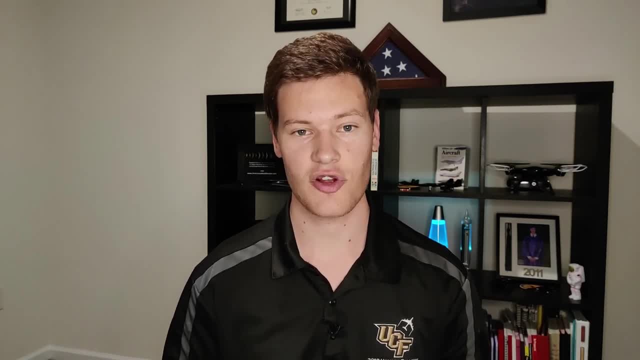 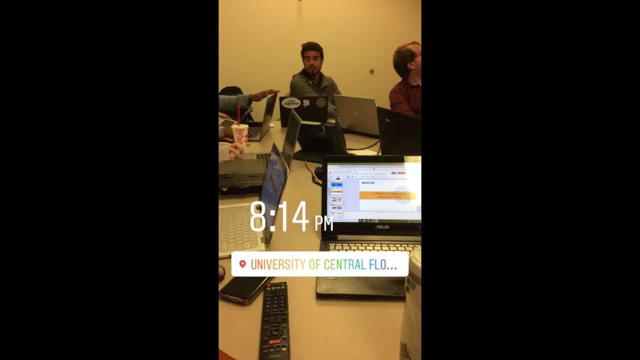 engineer, or actually any engineer in general- find a study group immediately. do it. your engineering course load is going to be absolutely insane. you're going to need a core group of friends that you can call each other to make sure you're doing assignments that you can study together. 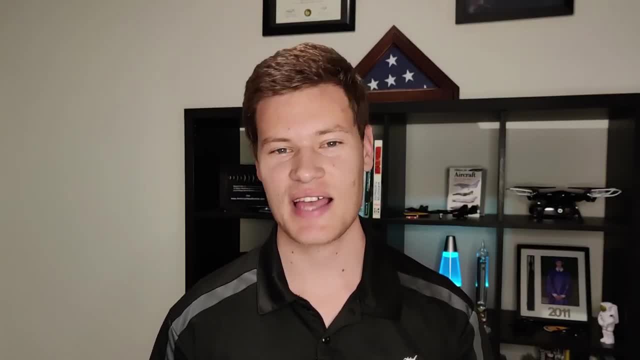 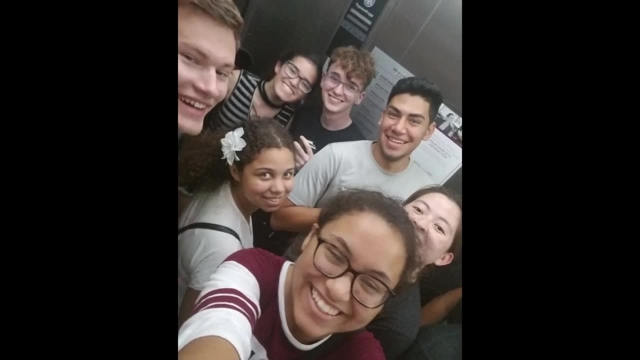 teach each other difficult concepts. it's been proven time and time again that studying in a group is vastly superior than trying to study on your own. not only are you going to be able to get help from your friends and explaining difficult concepts and helping you work through your homework. 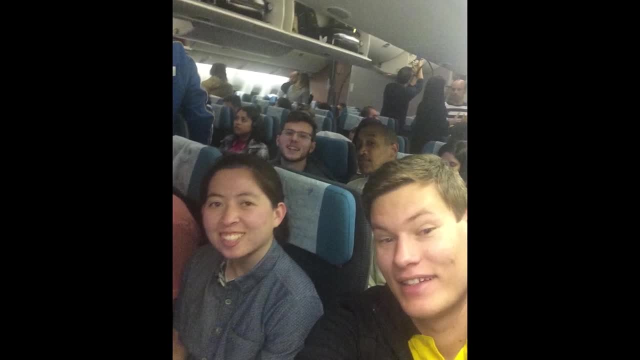 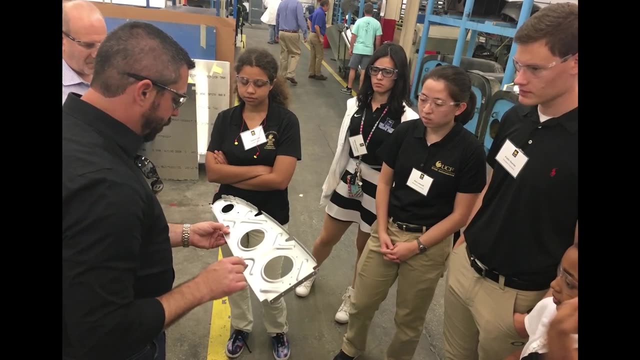 and studying. but even if you have a really good grasp on the content you teaching, it is going to reinforce it in your mind 10 times better. when you're able to explain a difficult concept to somebody in a clear and simple manner, you're going to start to grasp that concept even. 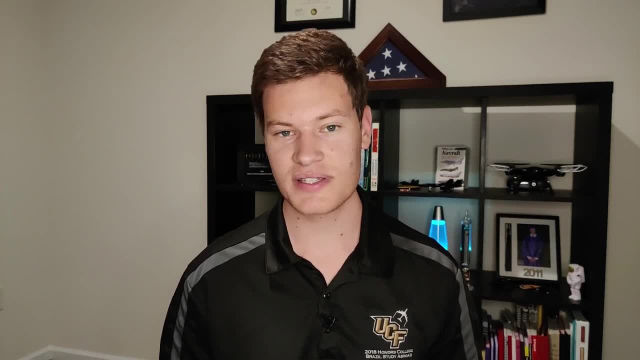 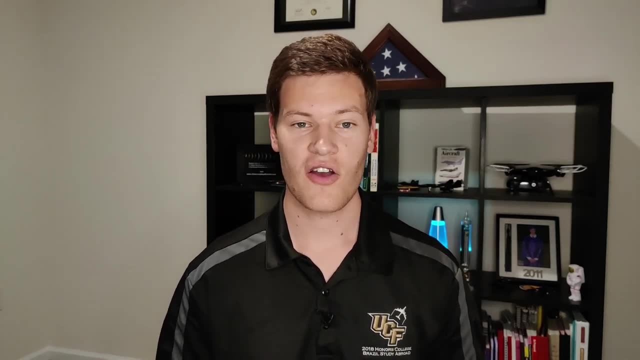 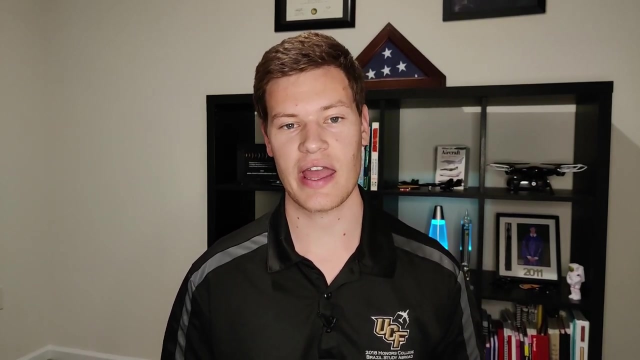 better than before. now. my next tip is probably the most important tip that i could give any aerospace engineering student for their time during college, and that is to get involved very early and very often in engineering organizations. now. the one that i would recommend is called ai double a. this 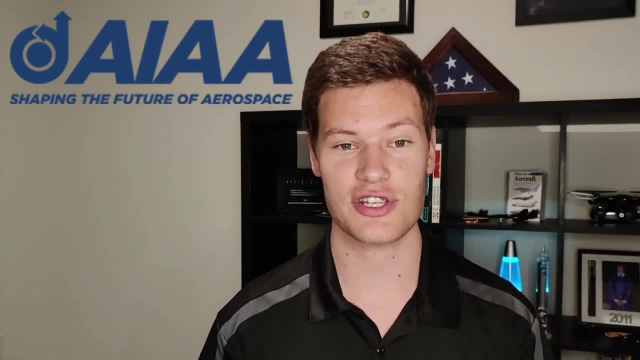 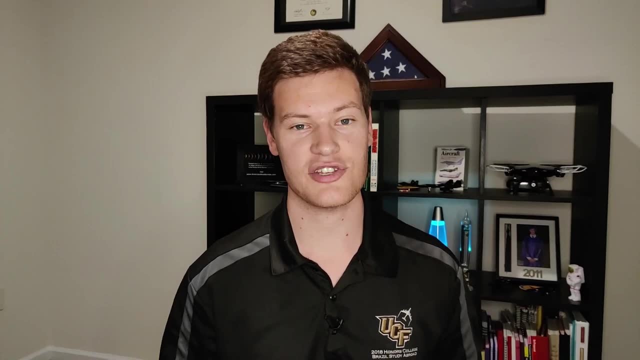 is the biggest and most widely known aerospace engineering organization and it would be very good for you to join the group if you're interested in learning more about aerospace engineering this organization very early. so the first reason that i always encourage people to get into engineering organizations early is because for one, they're just fun. for a lot of people myself. 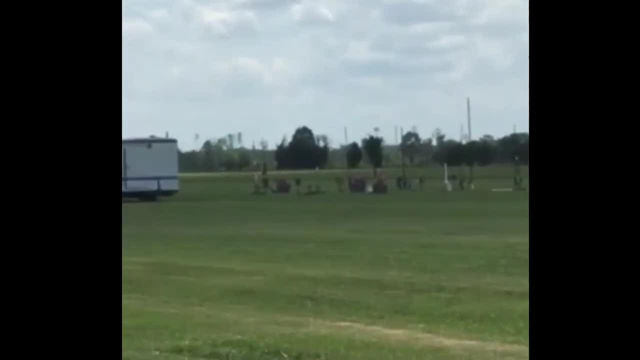 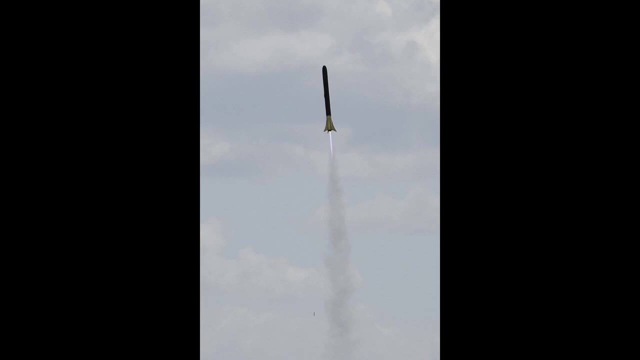 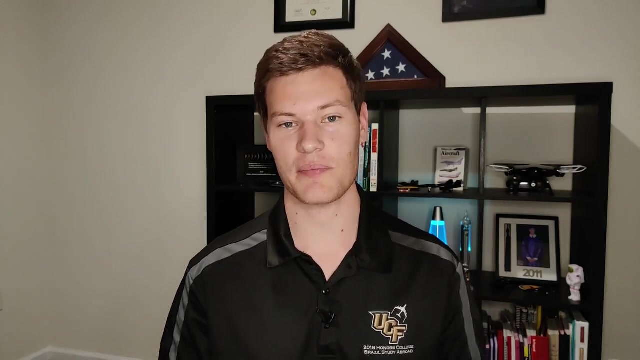 included. this is the first time that you're ever actually able to apply engineering principles into a real world engineering project. you get to put the principles that you're learning in the classroom into practice, into a real world scenario that you actually enjoy doing, and you actually get to build something out of it, and this can include anything from model. 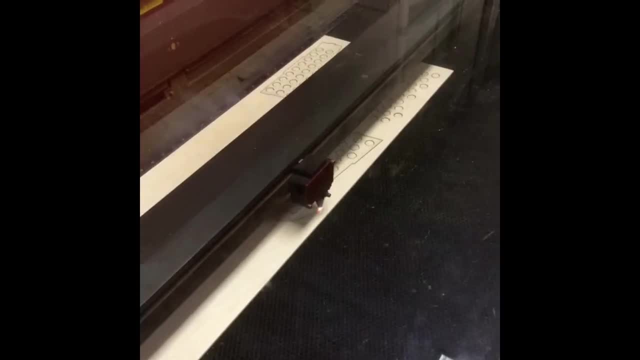 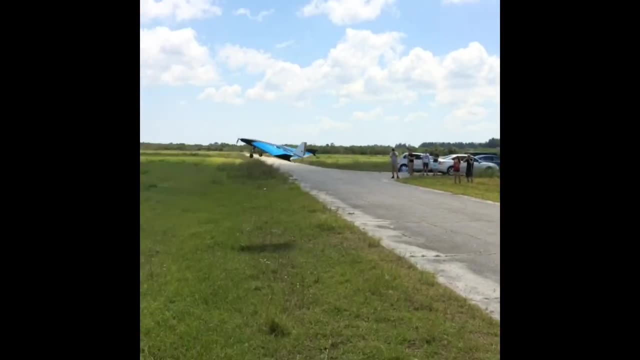 circuitry to building an airplane. not only that, but you're going to be put into groups with like-minded people, many of which you can form study groups because they'll be in your classes. the next, and probably more important reason that you should get involved in engineering organizations: 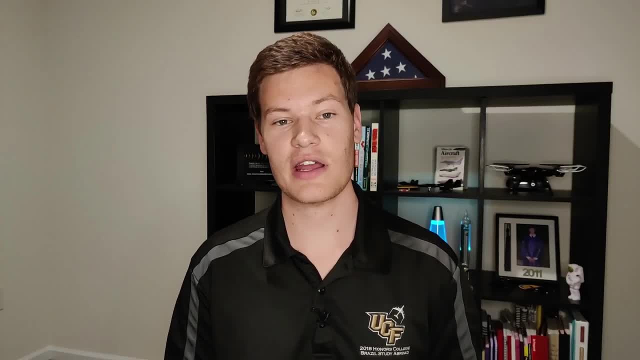 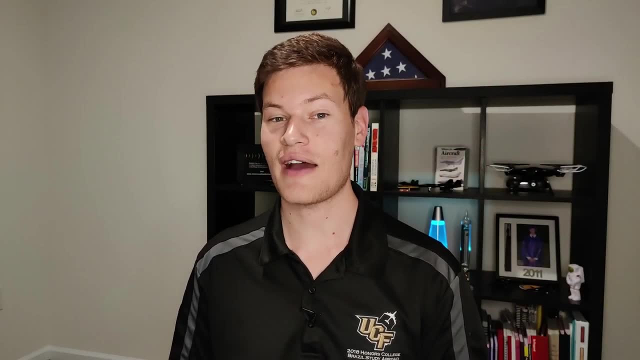 is because to get an engineering job you have to have experience, but to get experience you have to have an entry-level job. i'm confused, but that's why you have to do these engineering organizations. it's literally the only way that you can get into the industry. you have to have. 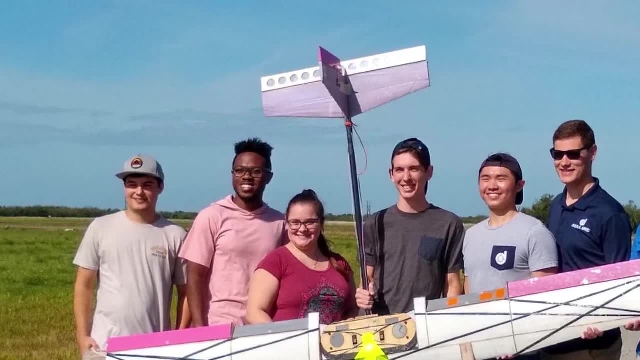 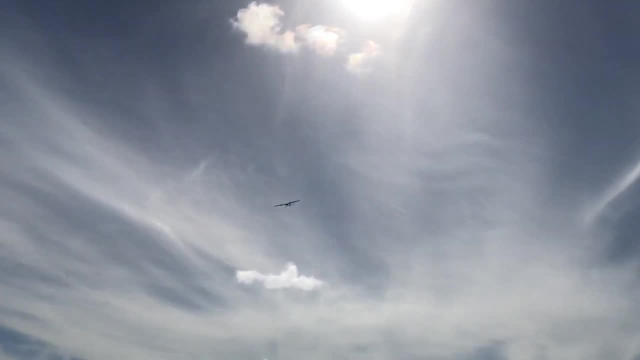 engineering experience and, yes, you can put these clubs and organizations on your resume because it does count as engineering experience. so, even though you may have never had a paid engineering position, when you're applying for an engineering job, you're going to have a full resume of these. 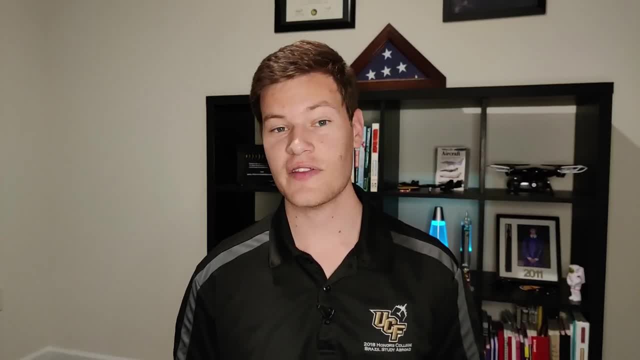 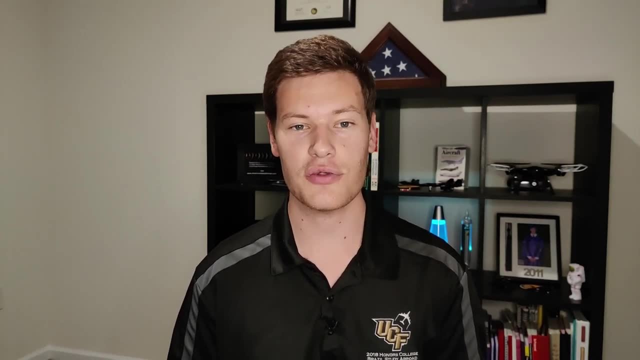 projects and these clubs and organizations. and this leads me to the next thing that you should always be doing during your college experience. when you're getting an entry-level job, it's almost entirely who you know, not what you know, because you're going to be competing with some of the most intelligent people that you've ever met. so one of the only 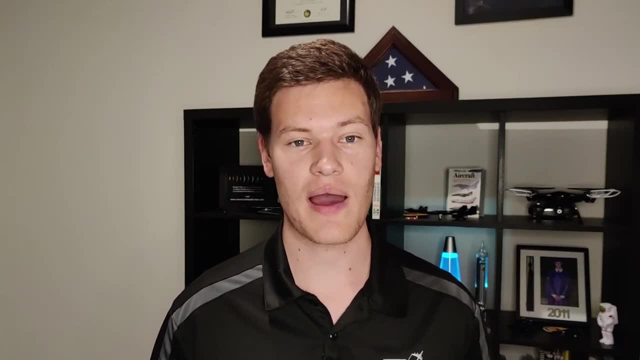 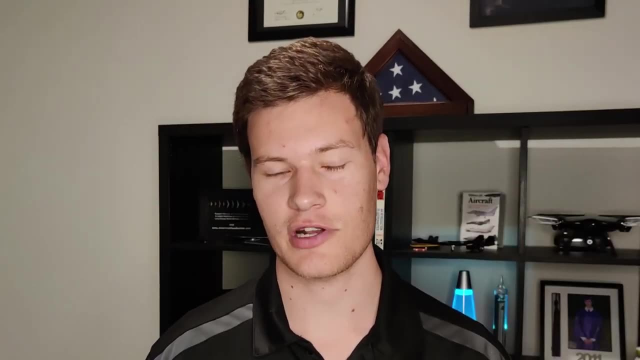 ways that you can make yourself stand out from your peers is to go out network, meet these people, get to know recruiters. add engineers on linkedin. don't just add random engineers, though they don't like that. make sure you know them first. you also need to make sure that you have a good resume. 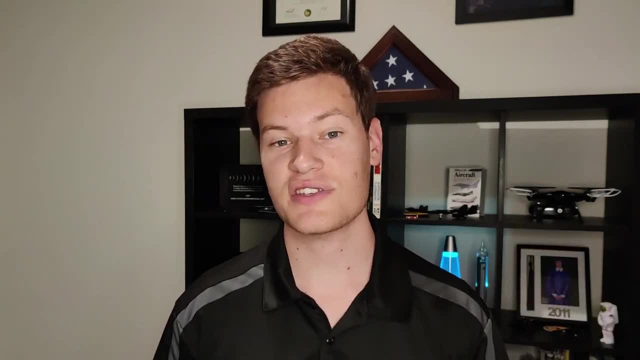 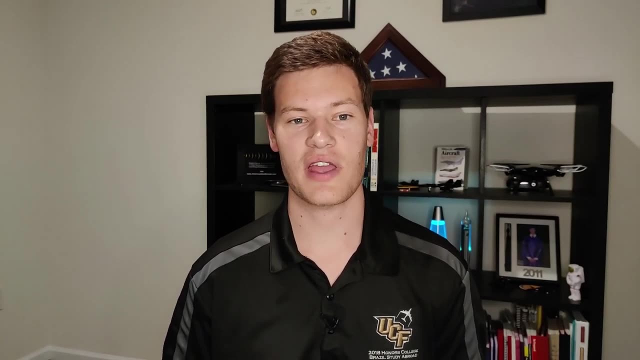 and you're always improving and updating it. most colleges have resources where you can go and get your resume checked for free. so utilize all these resources, but don't stop there. also get real engineers that you may meet in your community to look at your resume and critique you. i honestly 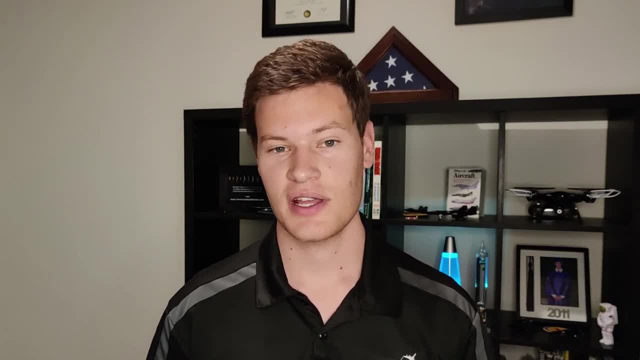 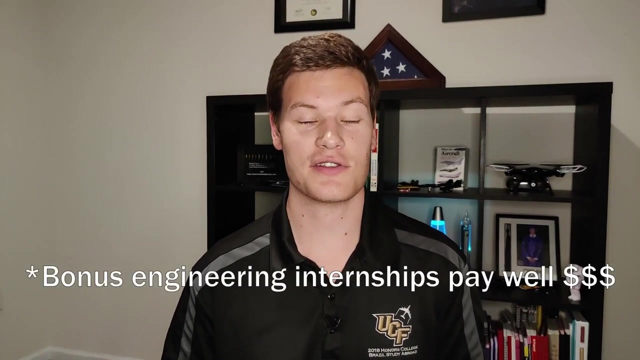 lost track of how many times i sent out my resume between jobs, getting people's critiques, getting people's feedback that i knew it had to be at least over 100 times. my next step for optimizing your time during your college experience is to get an internship and, like i said, to get an internship. 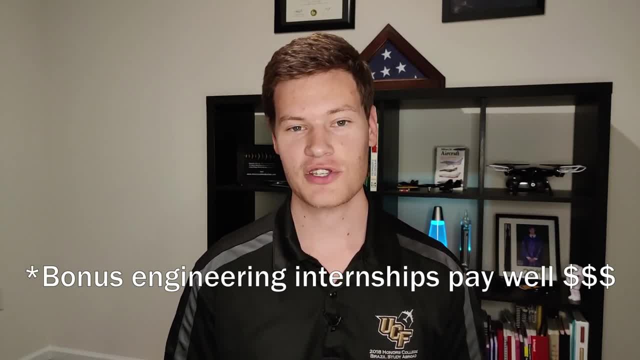 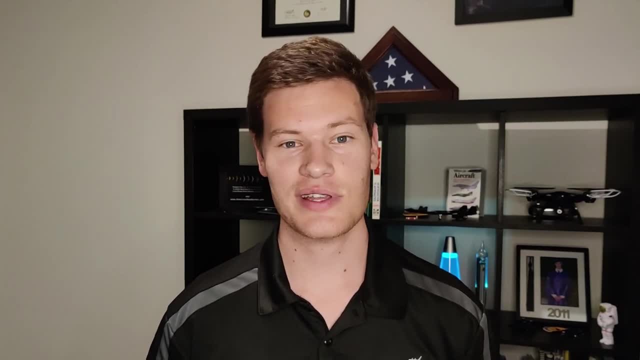 you really do already have to have engineering experience, which is where those clubs and organizations come back to the play. for me, getting an internship was incredibly difficult. in fact, i actually didn't get an aerospace engineering internship like i wanted. the only internship that i was able to get was 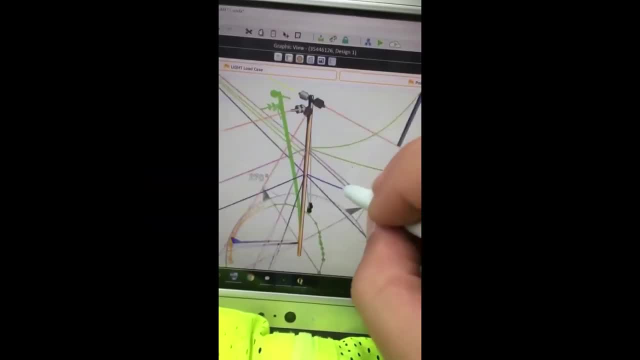 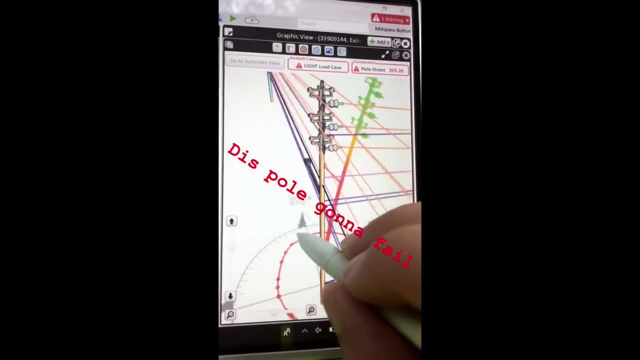 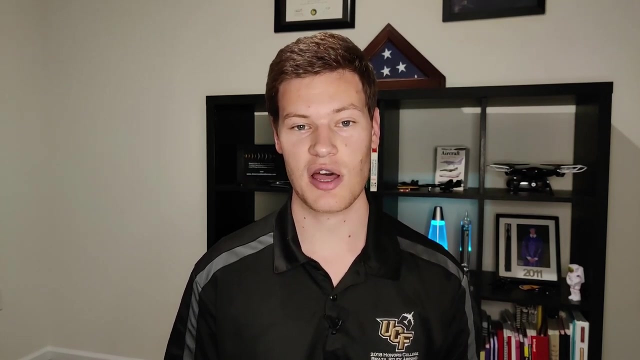 at a utilities contractor, but that was still my first experience with professional engineering and it was a great opportunity. not only are these internships good things that you can put in your resume when you're starting applying for full-time positions, but most of these internships can often lead to full-time positions at those companies. almost all my friends 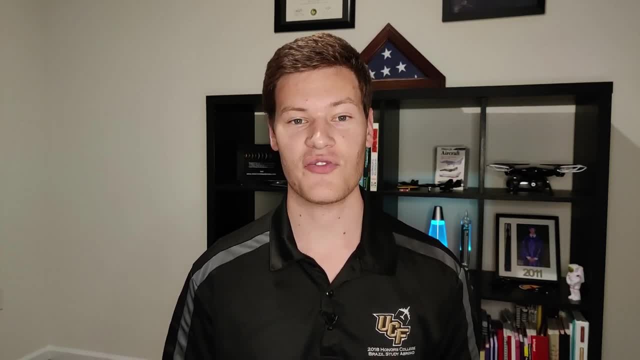 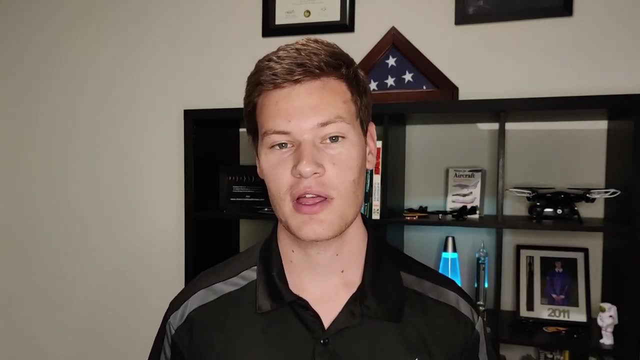 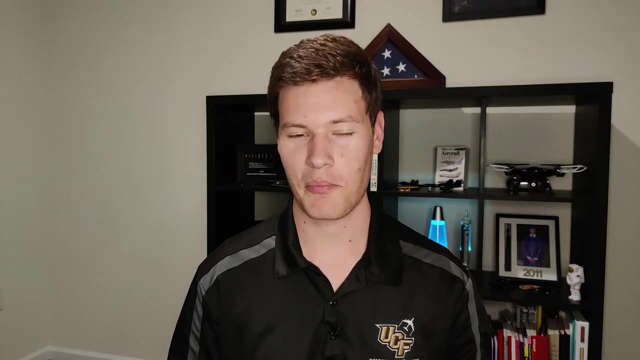 had internships at aerospace corporations, were offered full-time positions as they approached graduation, and the handful i know that weren't offered positions at the company after their internship ended up finding better jobs anyways. so now you're in your last year of your engineering program. probably your fifth year, but that's called being an engineer. but now it's time to start. 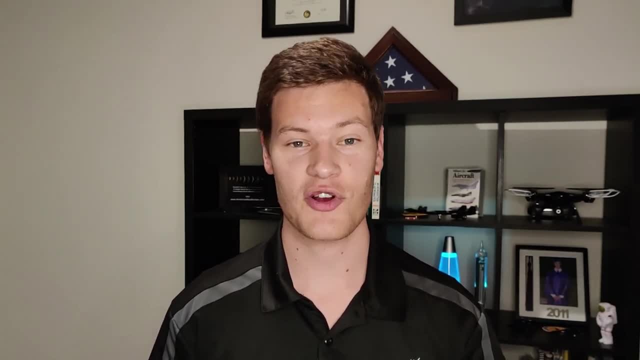 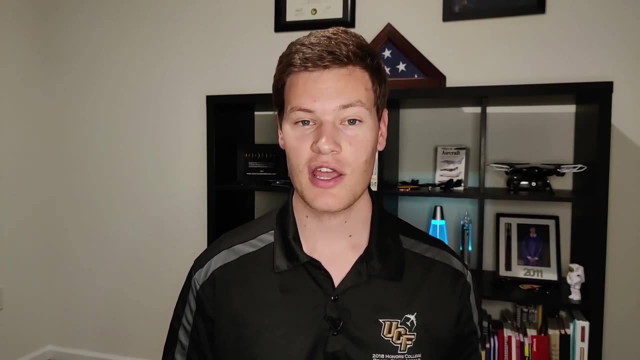 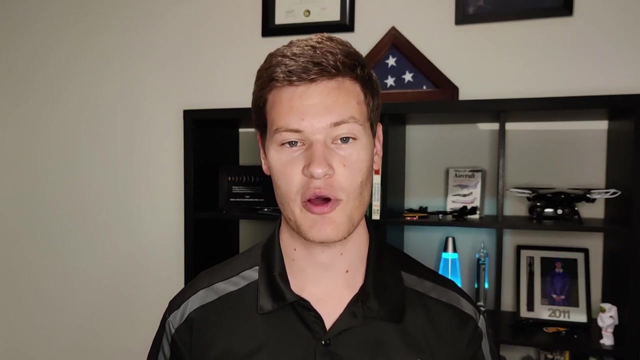 applying for jobs, and you need to start applying for jobs for a full-time engineering position at least two semesters before you graduate. that means if you're graduating in the spring, you need to start applying for jobs in the fall of that previous year. most aerospace companies in the us require that you have both citizenship in the united 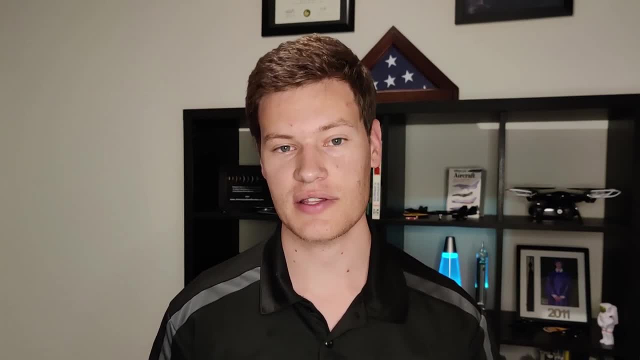 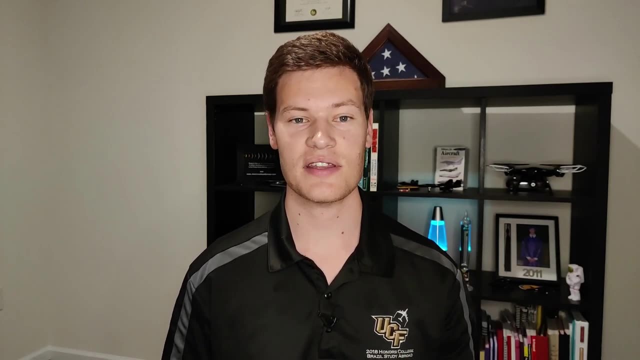 states and that you're able to obtain a security clearance. in fact, that's one thing you absolutely want to put on your resume if you're applying to aerospace industry corporations: that you're a us citizen and able to obtain a security clearance. for instance, i started applying for a job in september and i was offered the job in october of 2018 and i was graduating in may of 2019.. now applying for a job is very, very difficult. it really should be a part-time job- your senior year, after all. you're going to college to get a job, so don't forget that. 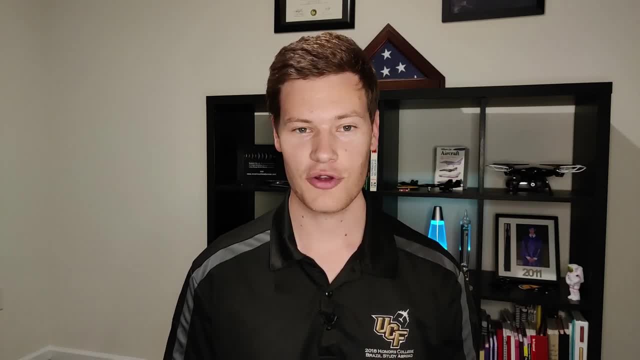 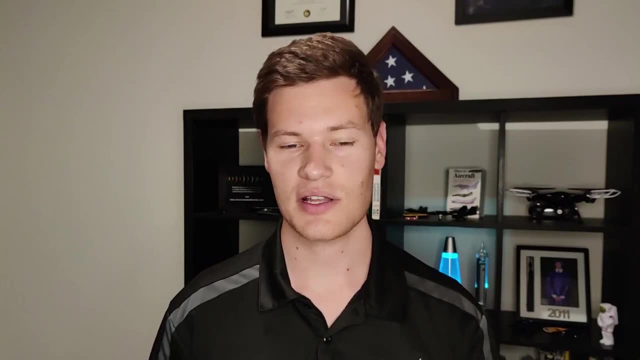 and just focus on whatever you have in front of you at the moment. you are in school to get a job, so just do it. make your dreams come true. i saw too many of my friends not focusing on getting a job, not putting in the effort, not applying all over the place. 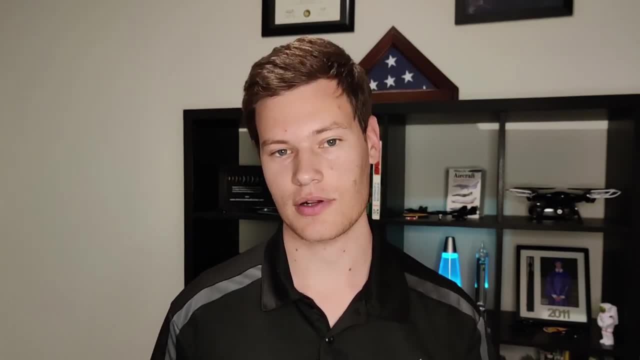 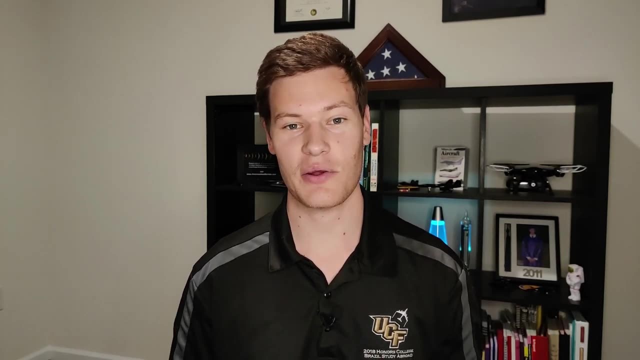 graduating, but then they didn't have a job until months afterwards. getting your first engineering job is really a numbers game. you're competing with thousands of thousands of the most intelligent people america has to offer, so, unless you're one of the lucky few that gets an internship during, your college experience and gets offered a full-time position after your internship ends, you're most likely going to have to apply for a ton of jobs. now there are a few shortcuts in finding these aerospace engineering jobs. so, like i said, i was not blessed with an aerospace engineering internship, so i had to work very hard to find my first job in the aerospace. 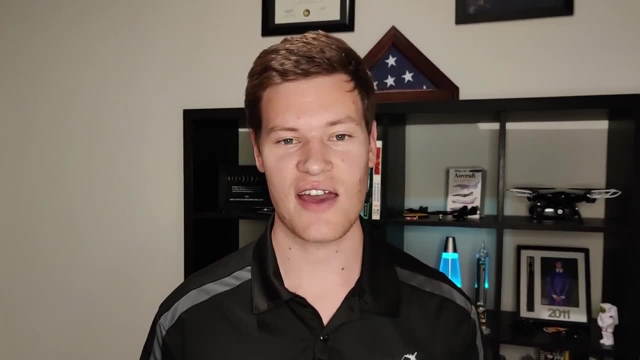 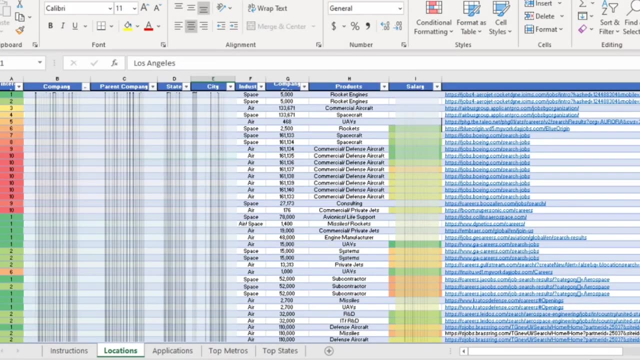 industry and as such, i developed a resource that lists every major aerospace company in america, that i could find what these companies do, what entry-level engineers get paid at these companies, based on data i could find in glassdoor where their locations are, how big the company is all. 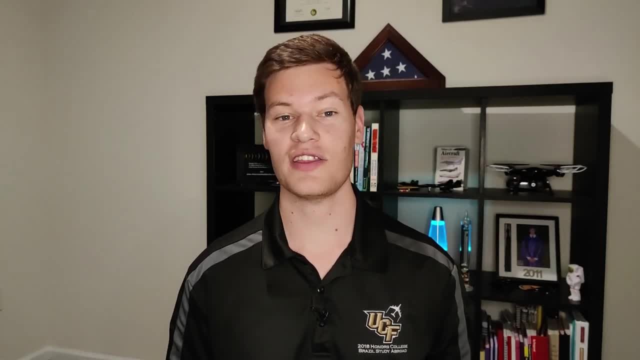 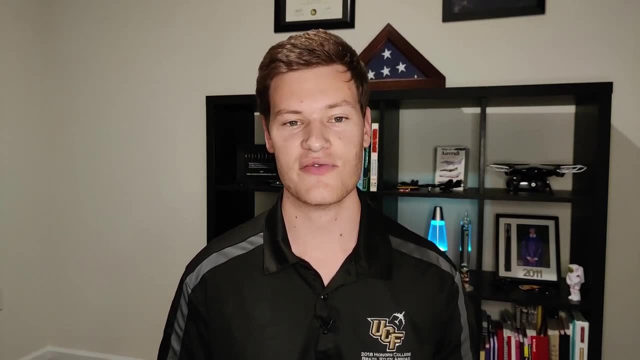 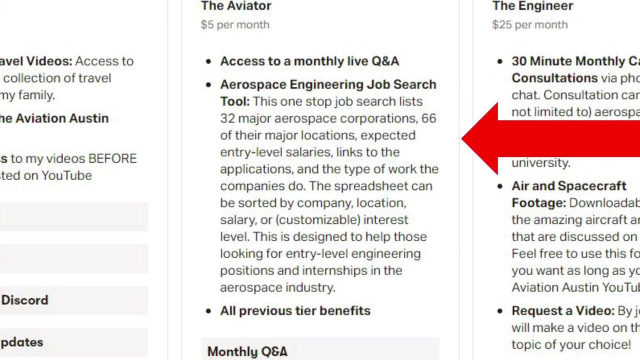 this information is in one resource and if you want a shortcut and you want to find all of these data that i've acquired in one resource where you can list all the resumes that you've submitted, all of the applications, the job recs, the statuses of these applications, all in one place, you can. 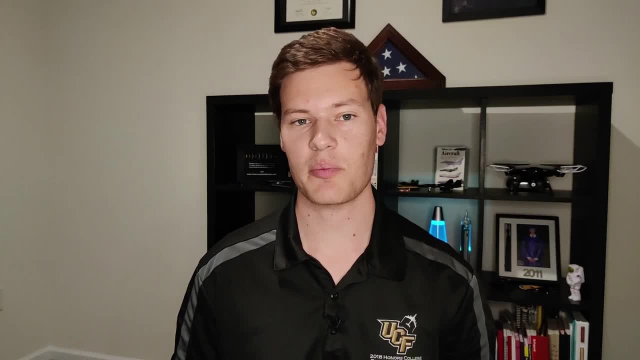 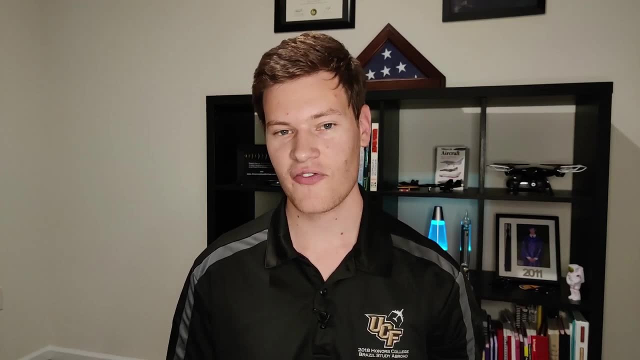 find that document in my patreon. so my next step in applying for an aerospace engineering position is: you want to make sure that every single resume that you submit is carefully curated for the position that you're applying for and unfortunately that's going to make the application process. 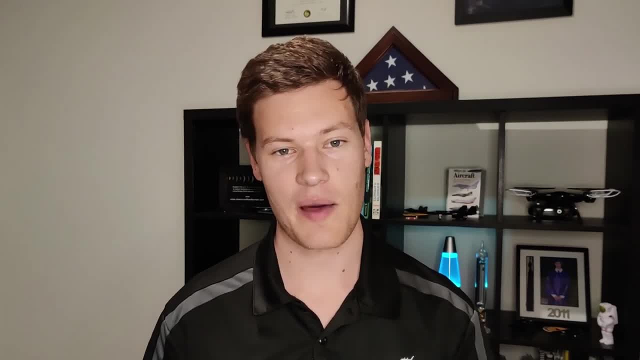 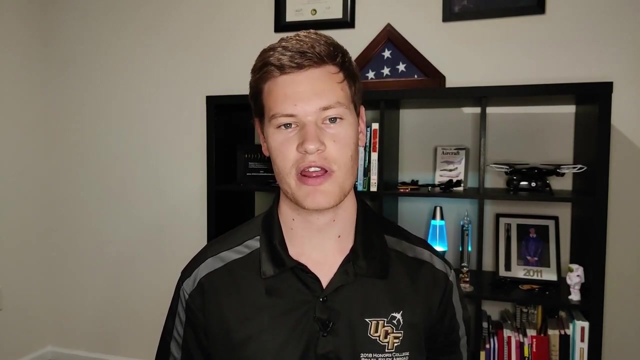 that much more difficult, because not only are you going to be writing all the applications and submitting the information for every single job, but now you have to actually write and rewrite your resume for almost every single position. now, the reason that you have to do this is because most big aerospace corporations 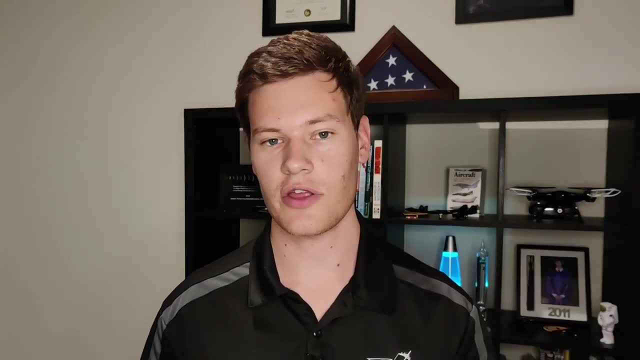 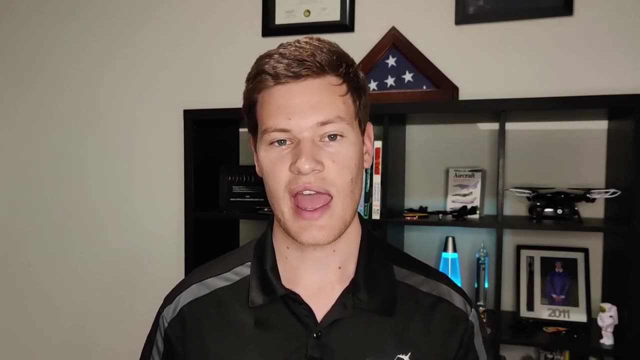 use a software to filter out applicants. so in other words, they put the keywords of what they're looking for in the job qualifications on the job description and they're looking for those keywords in your resume and if they don't see them, they go straight to the dumpster. so if you want to beat, 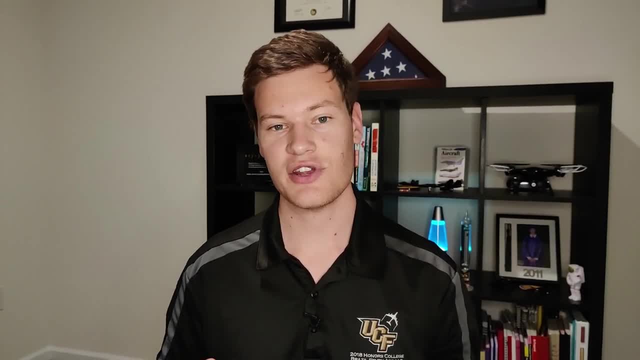 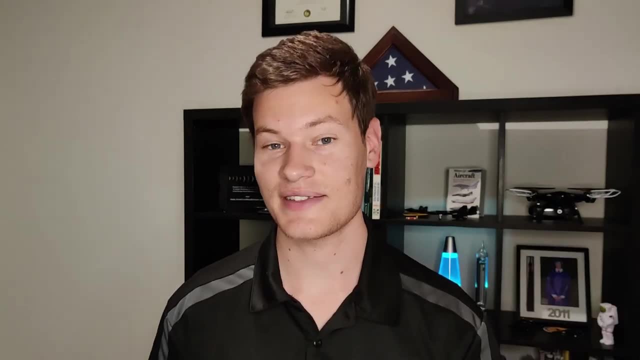 this software. you have to put those keywords into your existing resume or you're automatically going to get filtered and no human is actually going to ever see your resume. so, yes, it does suck, but it is important that you curtail every single resume that you put out there. 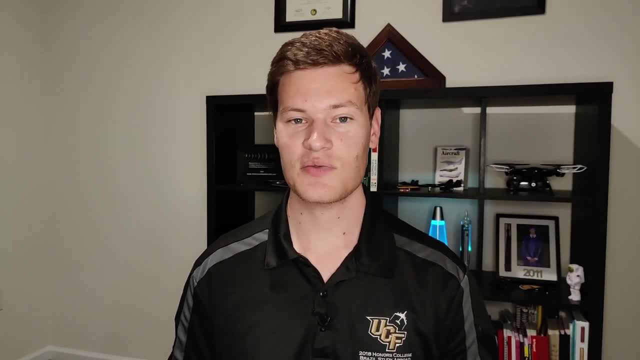 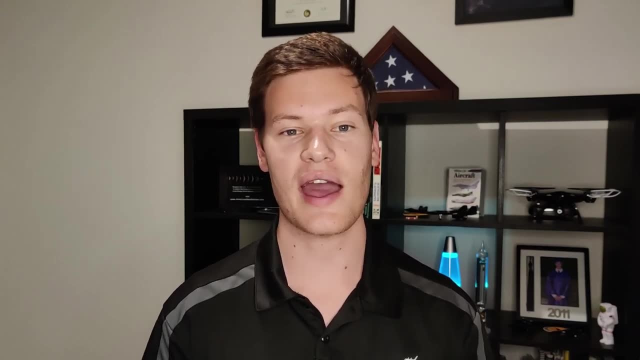 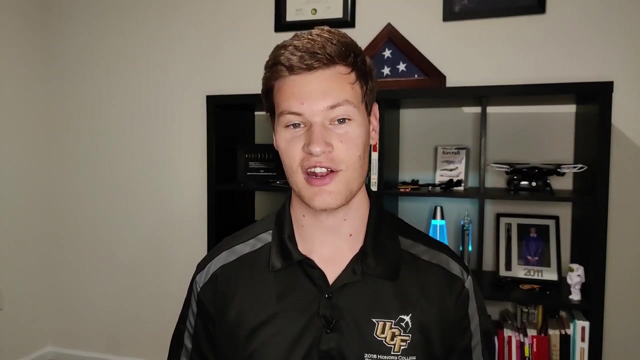 to the job description. now, there are some exceptions, and this is why it's so important to network. if you can successfully tap your network and get a recommendation from an existing employee in that company, they will pull your resume and bypass the computer entirely. that means that you're going to be that much closer to getting an interview and potentially getting a. 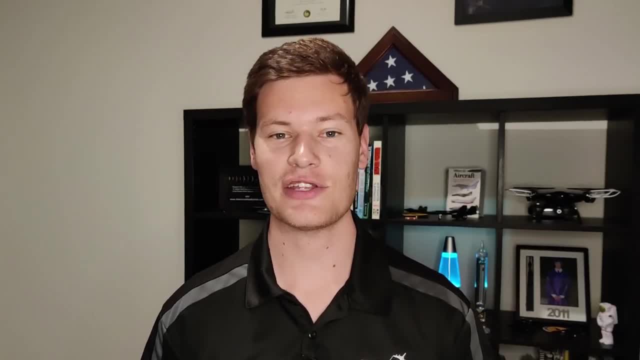 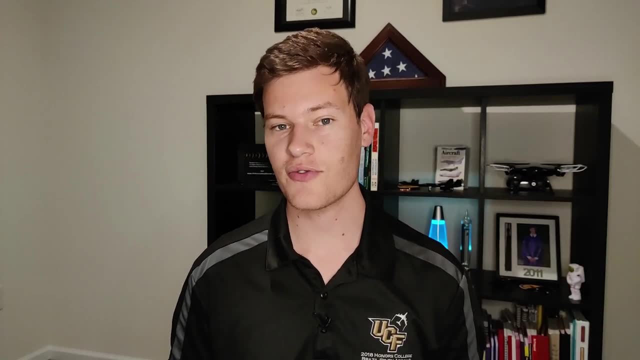 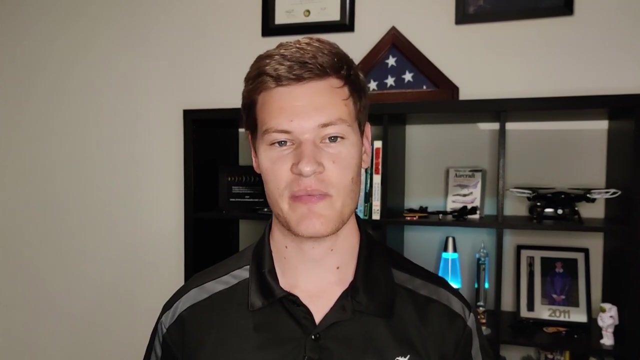 job offer for this organization, and one way that i haven't mentioned yet that is an incredibly powerful way to get a job offer is through conferences. conferences through major aerospace organizations are incredibly powerful resources. as an anecdotal example, i had several members of my senior design team go to an a processрown to investigate着old, but i realized that they 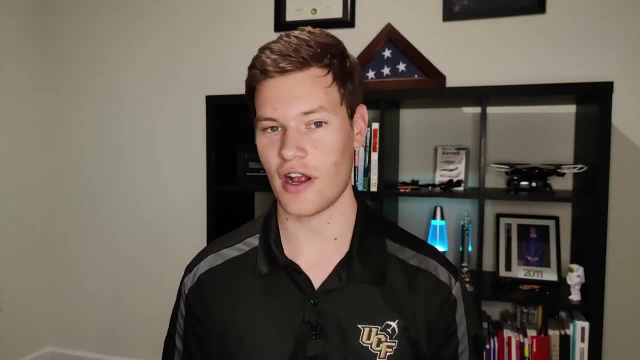 could learn a little bit more about the process. so i surprised everyone and taught them the next spicy. an example: i had several members of my senior design team go to an airspace program with a computer and ai double a conference their senior year. there was about five of them and a few of them already. 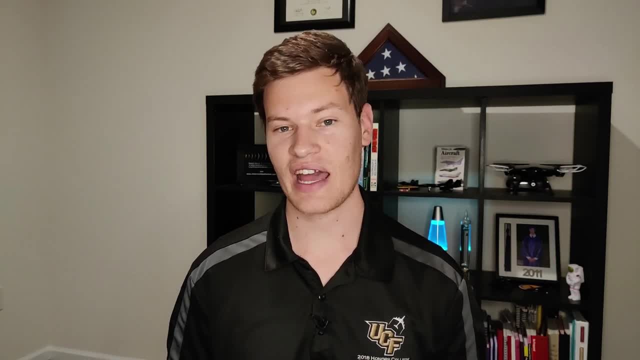 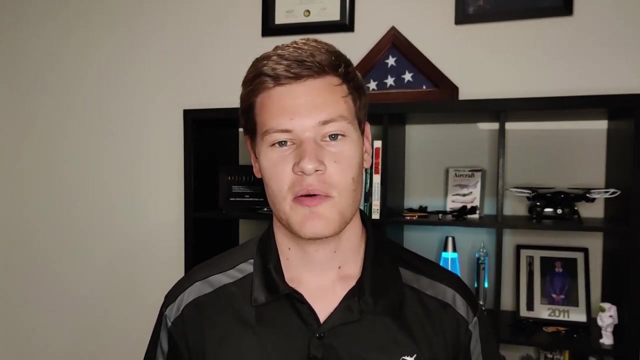 had job offers in hand, but the other ones that didn't already have job offers in hand- every single one of them that went there- was offered a job before they left that conference. and there are many conferences like this that you can attend and unfortunately, they often cost money. 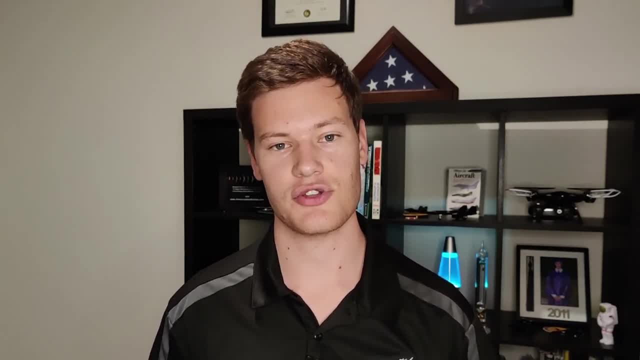 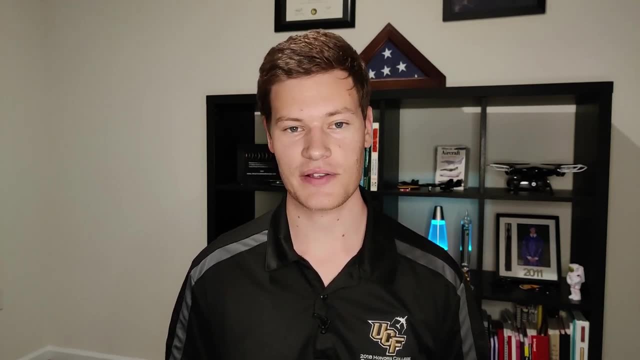 but usually they have a severely reduced price for students. so often these conferences will advertise prices like 500 to attend but the student price will be something like 50 bucks. and the fact that there are so many prominent engineers at these organizations and at these conferences, they really are 100 percent worth the cost of admission and if you're really strapped, 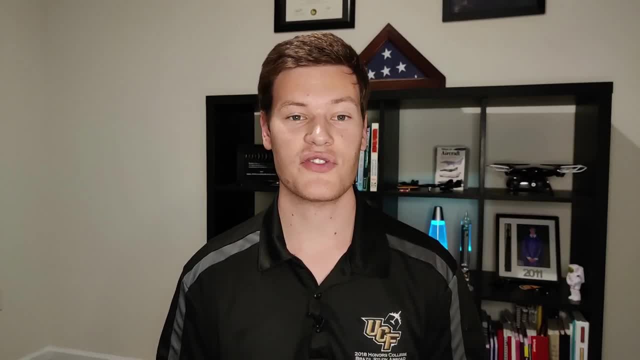 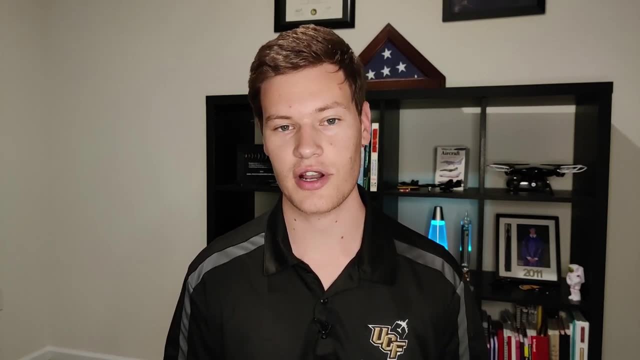 for cash and you can't afford to go to these organizations. there are often organizations at your school that will help you pay for this. for instance, at the school that i went to at the university of central florida, you could actually get it up to a 400 dollar stipend. 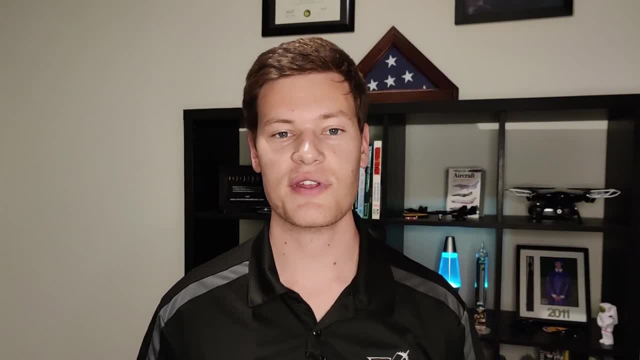 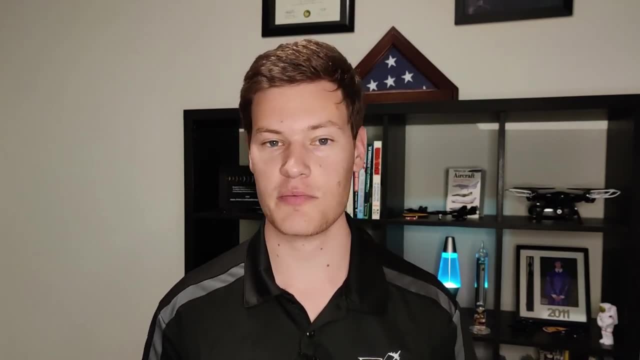 to attend these conferences. but, like i said, you're most likely going to have to apply for a ton of jobs. so make sure that you keep track of these in a spreadsheet like the one i offer on my patreon, or you can make your own, because you really don't want to get a call for a job that. 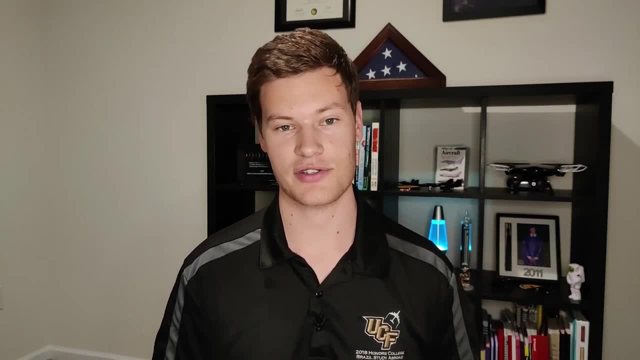 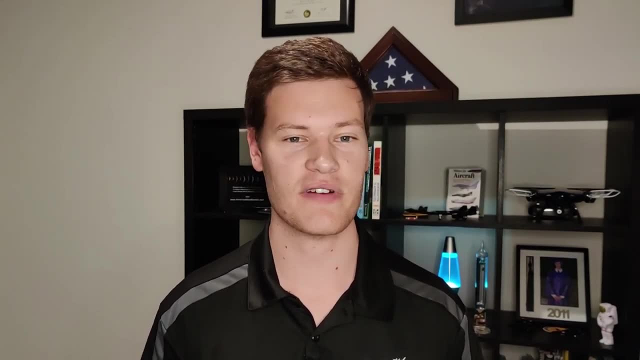 you don't even remember applying for and you're not able to find that job description. but, like i said, finding an aerospace engineering job is incredibly competitive. but don't lose hope. keep applying, keep putting your resume out there, keep networking, be active in these organizations and you can find a job. 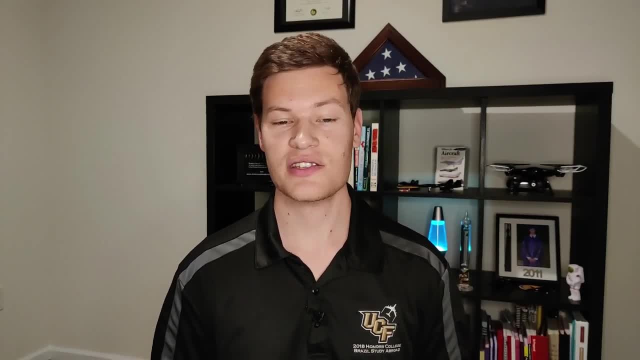 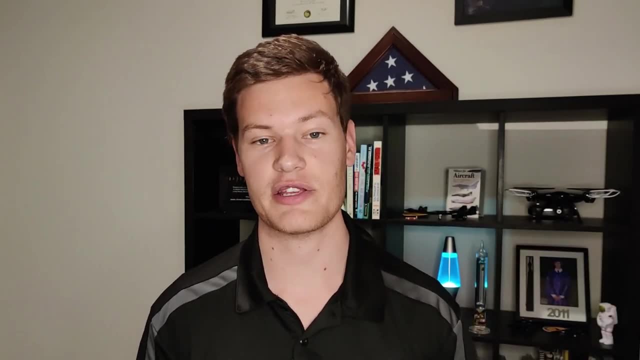 if it happens that you graduate and you still haven't found a job, this is just an opportunity for you to double down on your applications now, instead of going into your full-time position as an aerospace engineer. your new full-time position should absolutely be finding a full-time position. 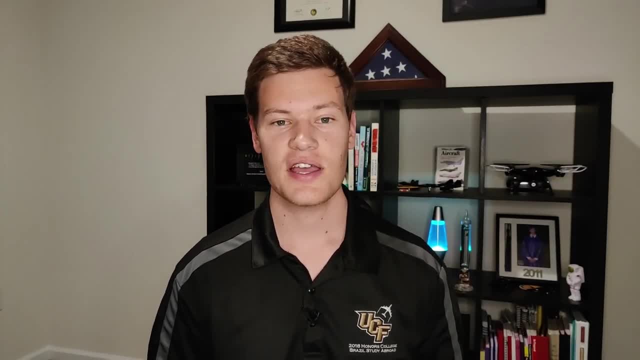 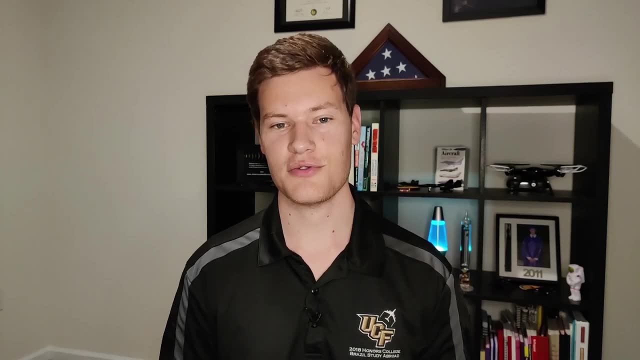 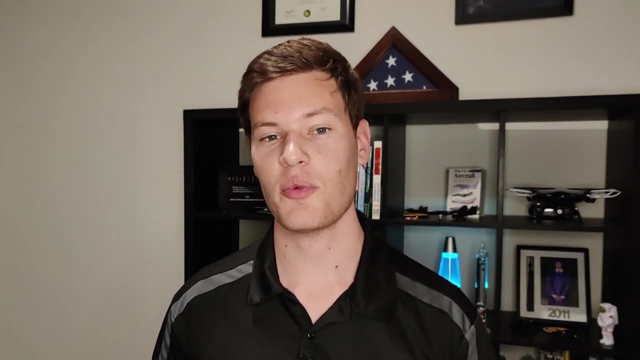 so keep going to these career fairs, keep going to these conferences, keep putting your name out there, emailing people that you know, recruiters, all these types of things. don't give up because you will become an aerospace engineer. so if you're at any of the steps that i've talked about in this video and you want personalized help with how you can,